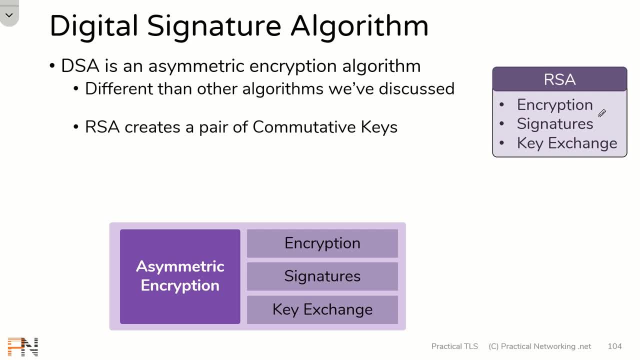 encryption by encrypting a message with the public key and sending it across the wire and the other side can decrypt it safely with their private key. We can use RSA for signatures by doing sort of the inverse: We can hash the message we want to sign, encrypt it with our 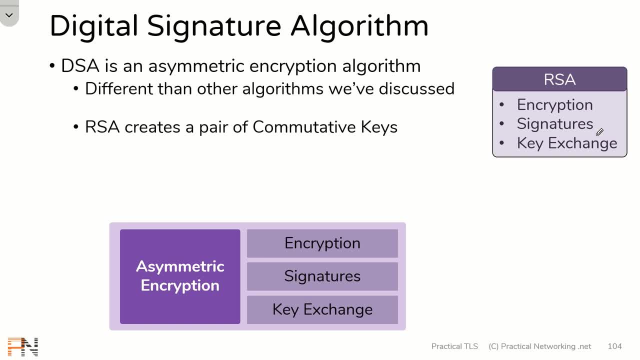 own private key and send it across the wire And the other side can validate the signature with my public key. We can also use RSA to do a key exchange by using the encryption mechanism we just discussed to send across a seed value to generate keys, So RSA can. 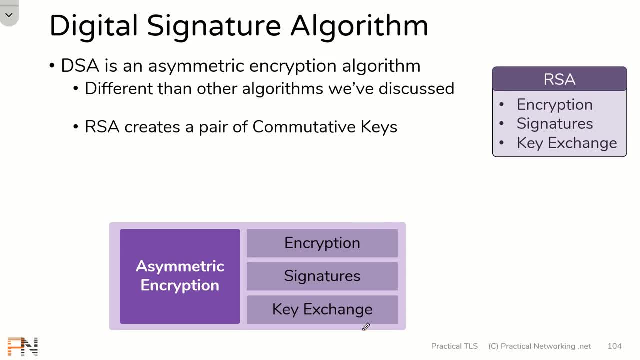 be used for all three of these asymmetric encryption functions. Now we also talked about the Diffie-Hellman protocol. We discussed that Diffie-Hellman can be used to establish a shared secret over an unsecured medium. With this list over here, that means that Diffie-Hellman can only be used for this function. 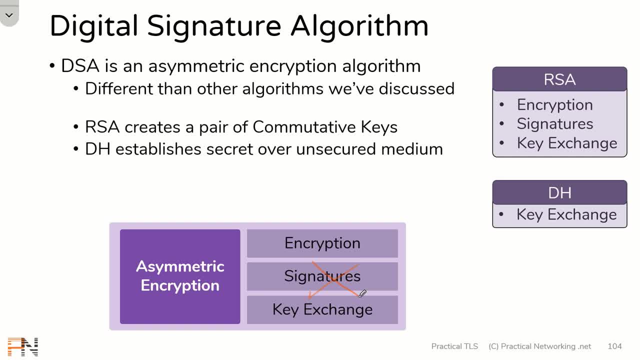 We can't do encryption with Diffie-Hellman and we can't do signatures with Diffie-Hellman, Which finally brings us to DSA. DSA is another asymmetric encryption algorithm, but it can only be used for signatures. It can't do encryption and it can't do key exchange. That is the. 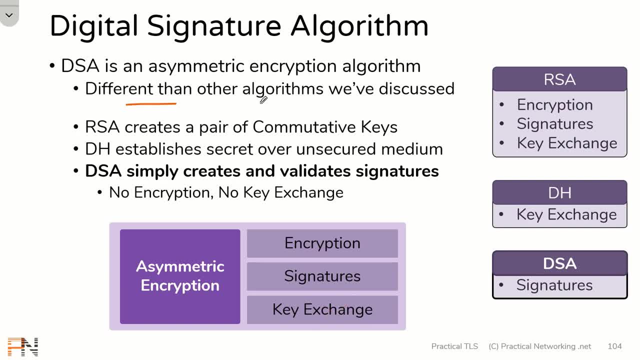 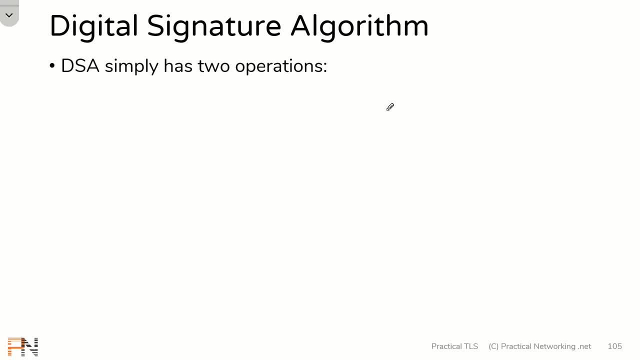 digital signature algorithm And that's how it's different from the other algorithms we've discussed. So the digital signature algorithm is an asymmetric encryption algorithm with only two operations: Signature generation and signature verification. The signature generation operation involves four things: The message you're trying to sign. the private key you're going. 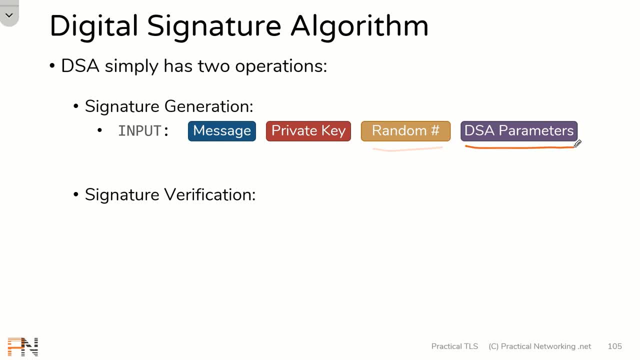 to sign it with a random number and these DSA parameters. These DSA parameters are values which are required for the DSA math, much like the prime number are values that are required in Diffie-Hellman. Either way, if you feed these four things into the signature generation operation, DSA. 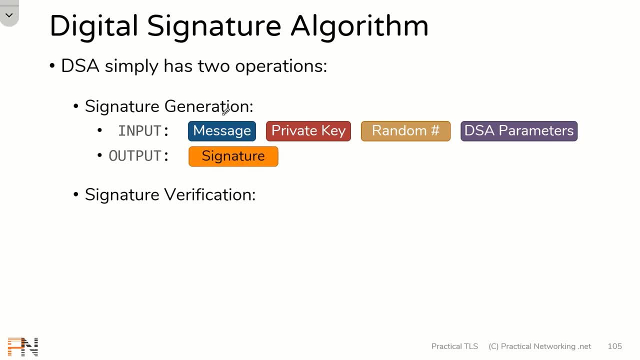 is going to spit out a signature correlating to that message, Then the signature verification operation also requires four things: The message you're trying to verify. the public key which correlates to the private key which was used to create the signature. the signature itself. 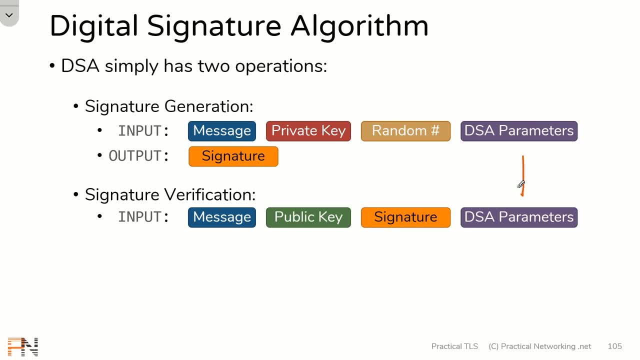 which was the output of the signature generation operation, and then, finally, those same DSA parameters. If you run these four things through the signature verification operation, DSA will spit out a 1 or a 0, indicating true or false meaning. is the signature valid or invalid? 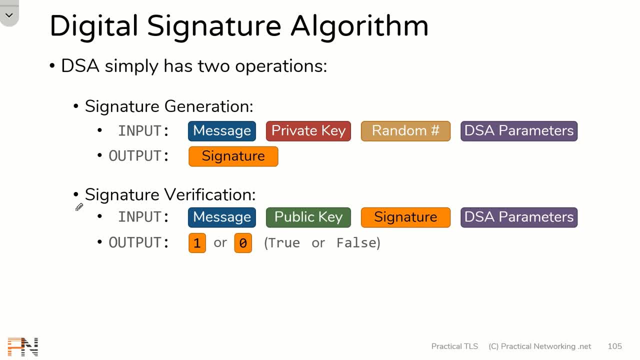 That's it. Notice, there's no encryption, there's no ciphertext, there's no plaintext. All you can do with DSA is generate signatures and verify signatures. Notice, that's sort of baked into the name. It is simply a signature algorithm. Now I want to talk in more detail about something. 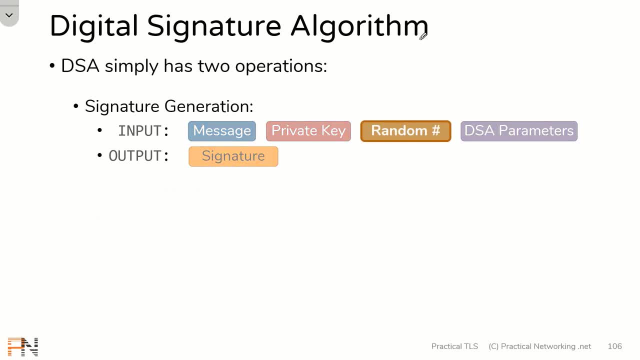 important about the DSA algorithm. It has to do with that random number. That random number is very important. It must be unique for every single message that you're trying to sign, or DSA will fail catastrophically. What I mean by that is if you happen to reuse. 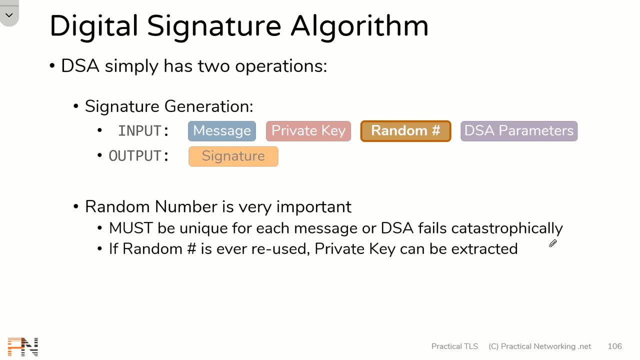 that same random number on two different messages. you can compare the signatures of both of those messages and extract the private key. That's really bad. That's why DSA can fail catastrophically if you don't use your unique signature. That's the whole problem with. 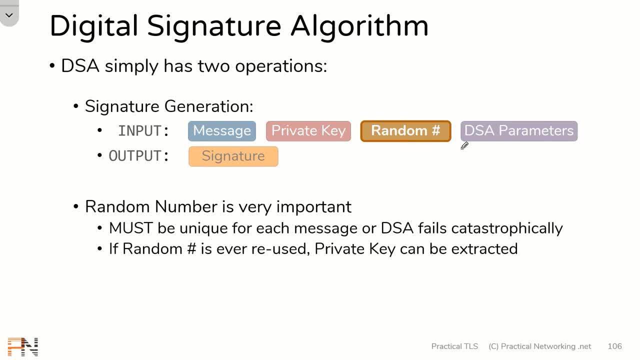 DSA random numbers. One option is to use a random number that is so large that you never run the risk of using the same random number twice. Another option is to use RFC 6979.. This RFC allows you to deterministically generate a random. 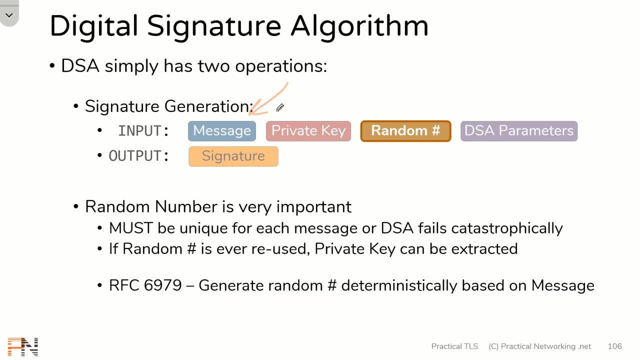 number based upon the message you're trying to sign. What that means is, if you use the formula outlined in this RFC, the only way you'll ever have duplicate random numbers is if you're trying to sign the same message, and if that's the case, you don't have this failure point because either way, you're signing the. 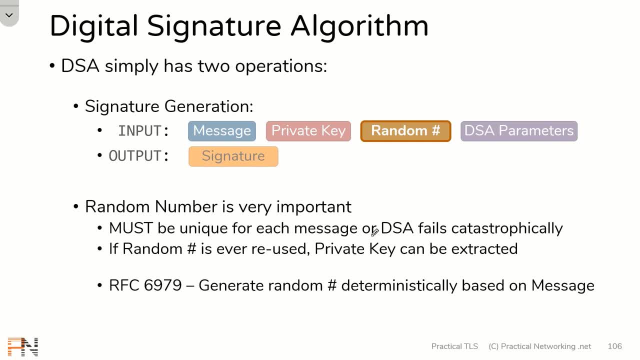 same message. So that's the digital signature algorithm. Now we're not going to actually go through the math for DSA. The math is actually pretty complicated, much more so than it was for Diffie-Hellman and RSA, which we did do the math for The 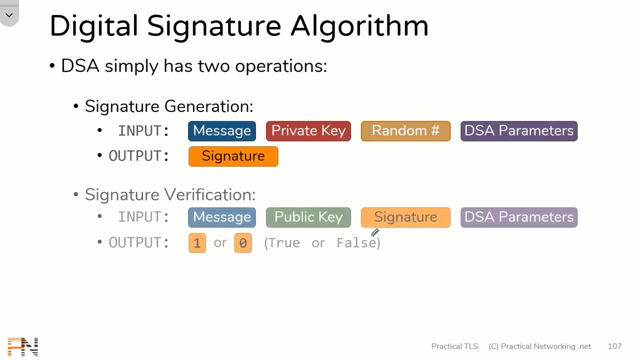 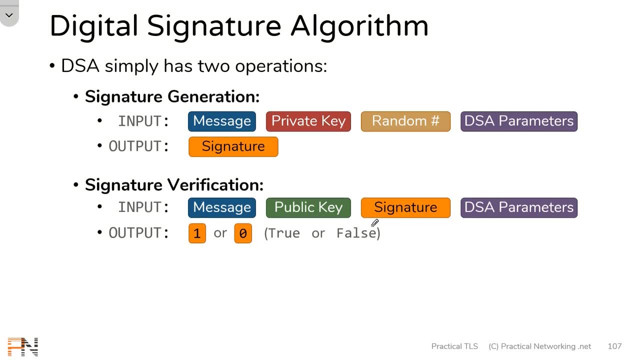 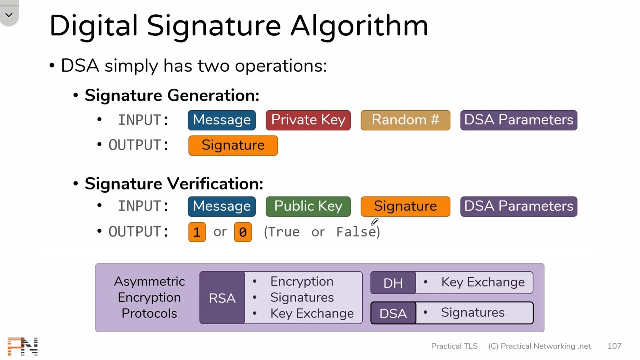 main things to understand about DSA is that it is an asymmetric encryption protocol that can be used for only two things: signature generation and signature verification, And understanding how it is different from the other asymmetric encryption protocols that we've already discussed. So that's it for this lesson. The main takeaways about DSA are on your screen. 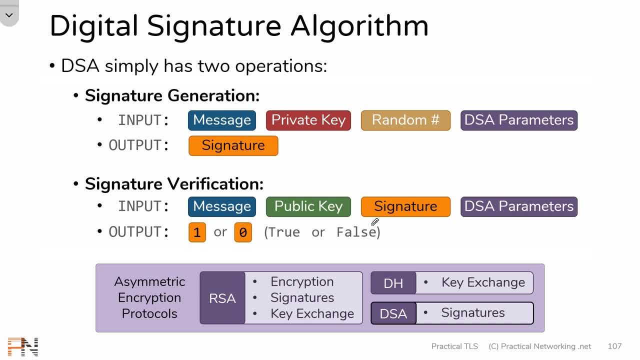 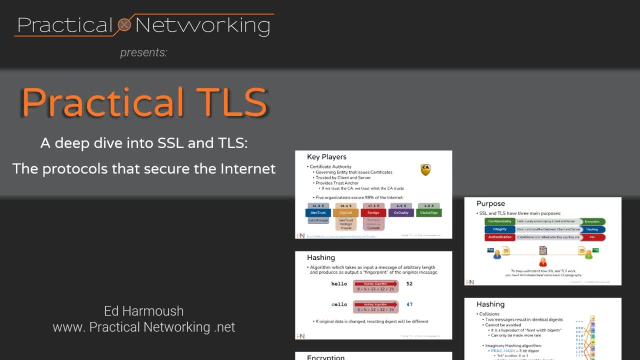 right now. I hope you enjoyed this video. I want to thank you for watching and I'll see you in the next one. Hey, YouTube, if you enjoyed that lesson, then you'll also enjoy the full course that it came from Practical TLS. It's a deep dive into SSL and TLS taught.